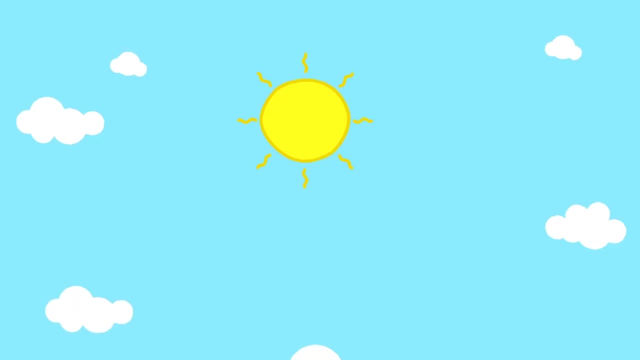 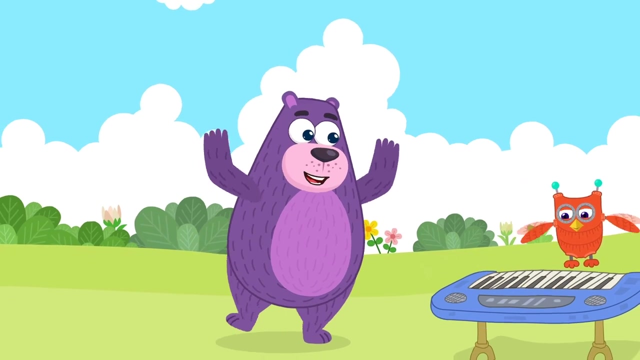 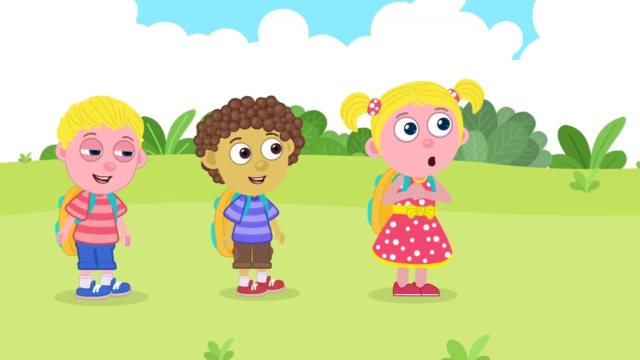 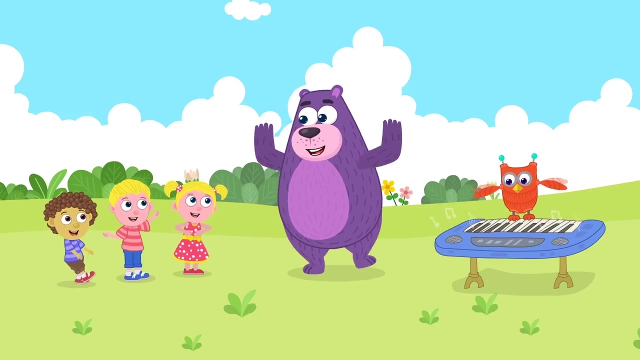 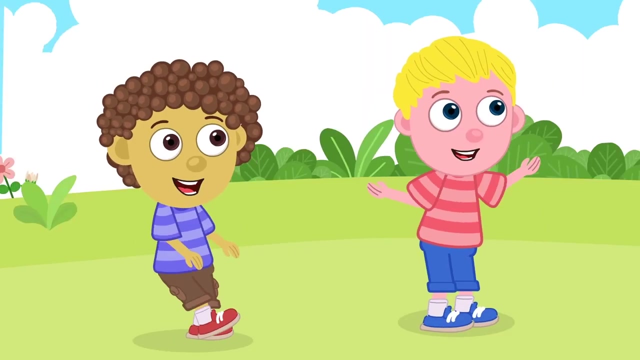 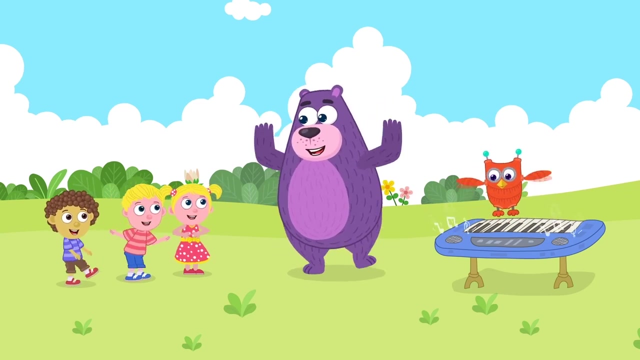 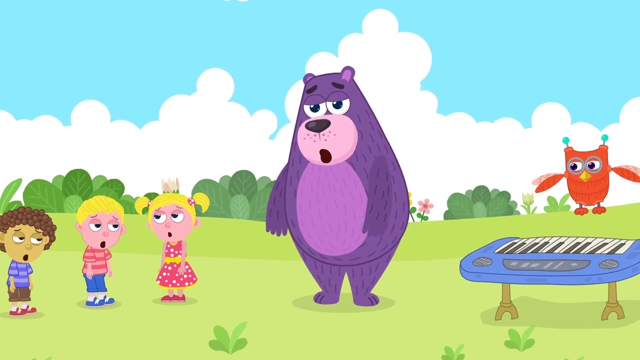 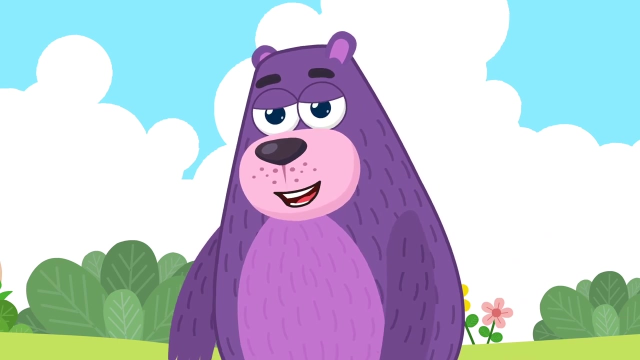 Polly seems to be in a good mood today, and it's no wonder. The sky is blue, the fields are green and lush. Life on planet Earth is beautiful. Oh, I love dancing. Come on, boys, let's join in. That was so much fun, but tiring too. Who needs a drink and a snack? 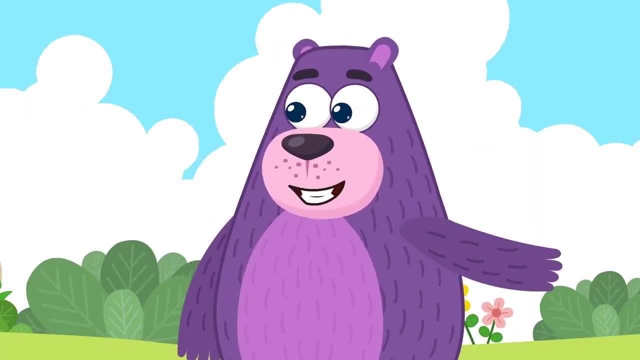 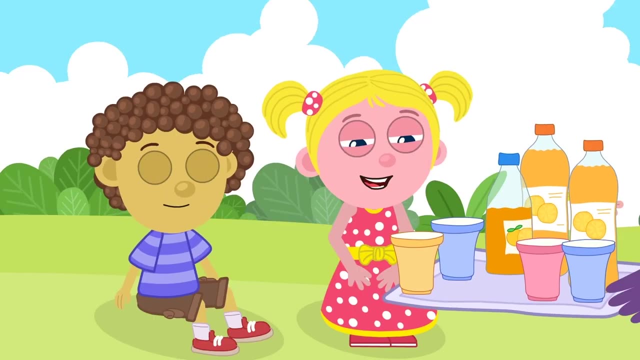 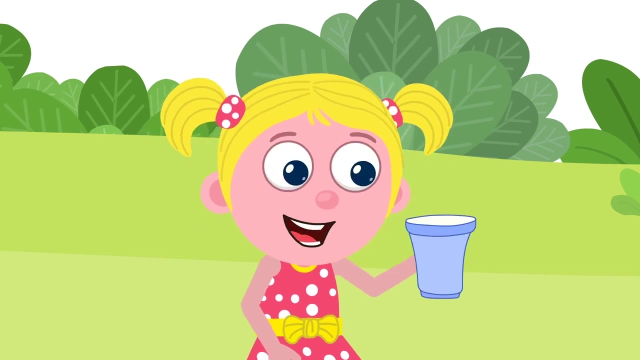 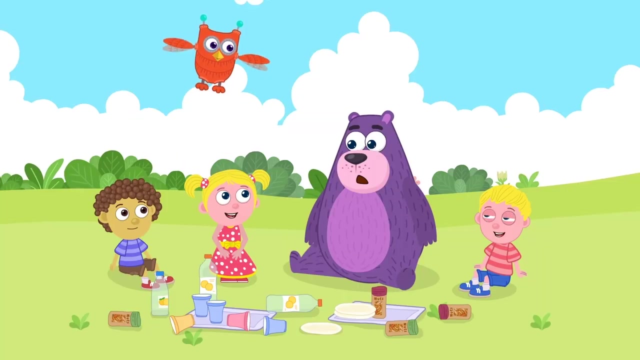 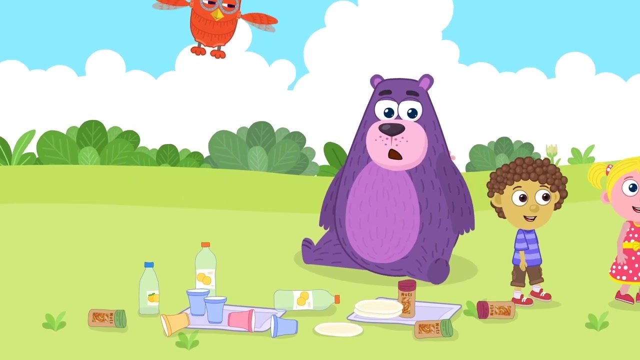 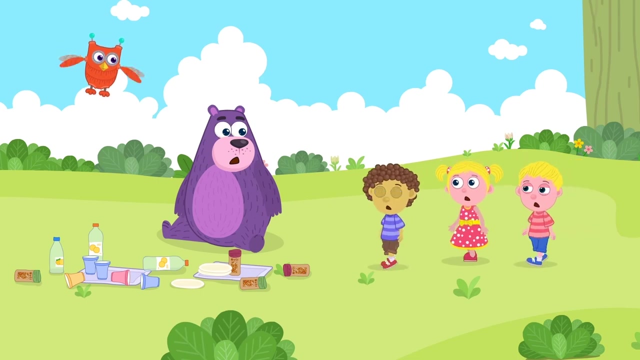 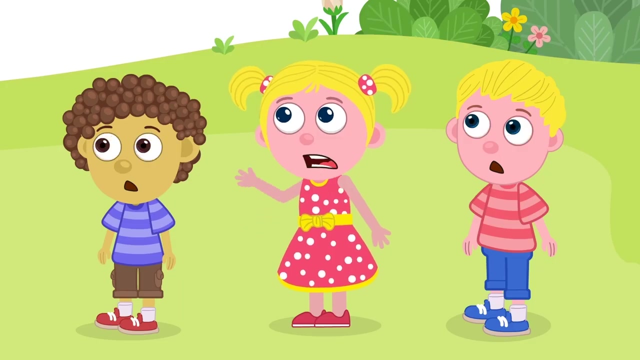 Me too. I'll go and get some from the treehouse. Yeah, Finished, We're ready. Olly, Can you play some more music? Future Danger. What's wrong with Ollie? He's worried about the planet, The planet, But why? 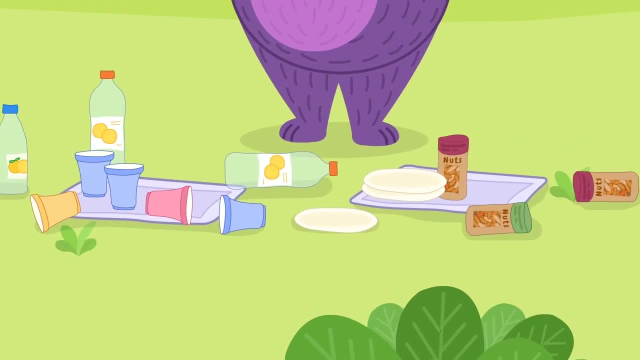 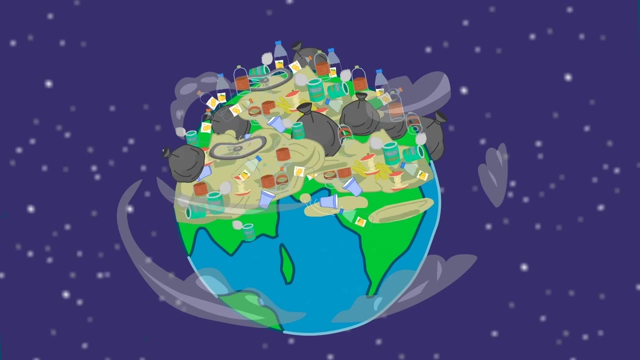 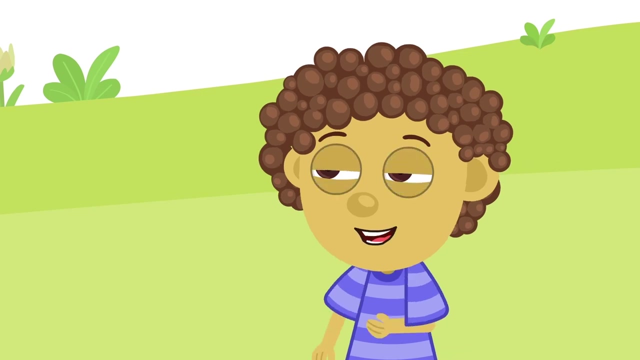 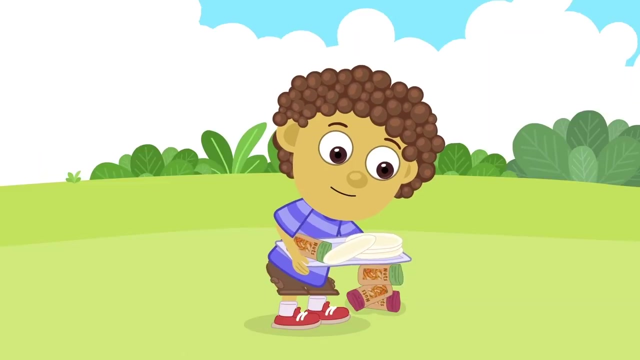 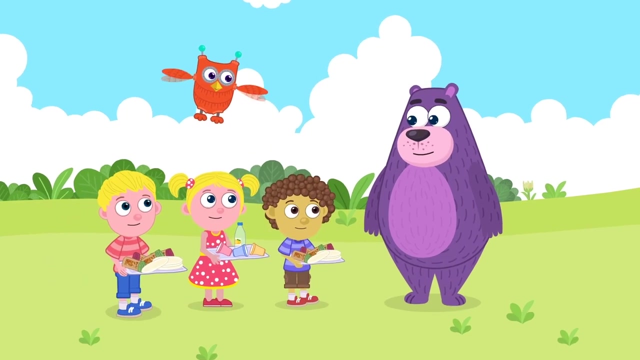 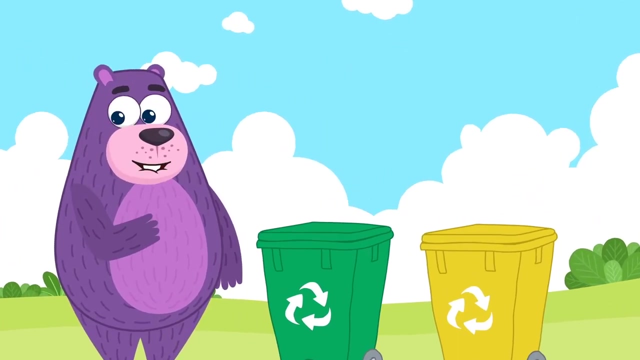 Because of all the rubbish you've left. If we don't recycle, the Earth will be full of rubbish mountains. Sorry, Polly, Sorry Ollie. We'll recycle our rubbish right away. Where's the bin, Polly? We have more than one bin. 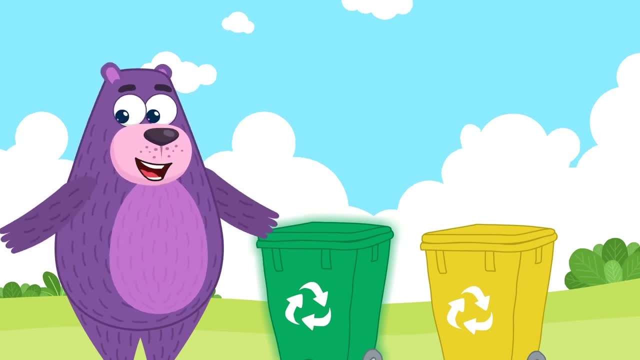 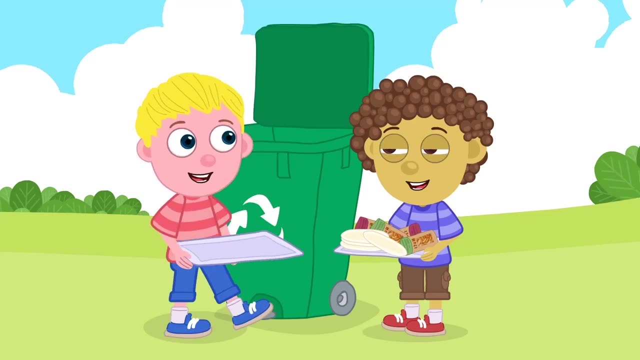 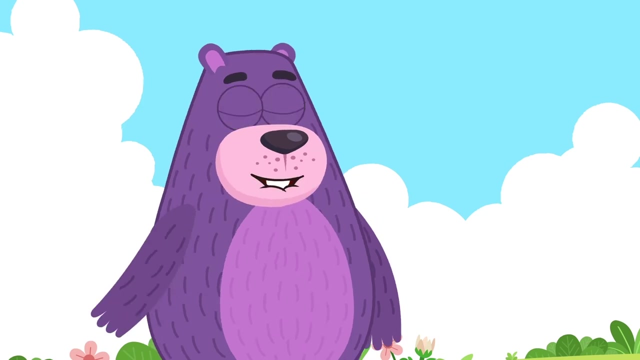 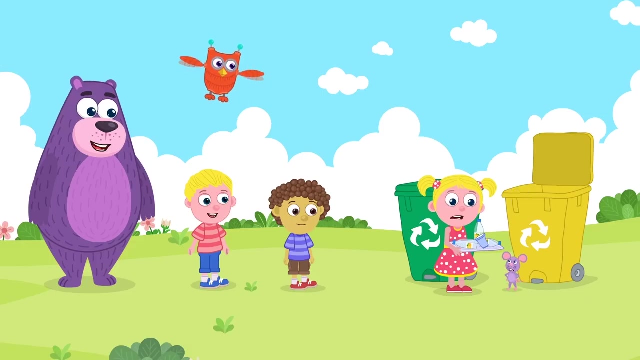 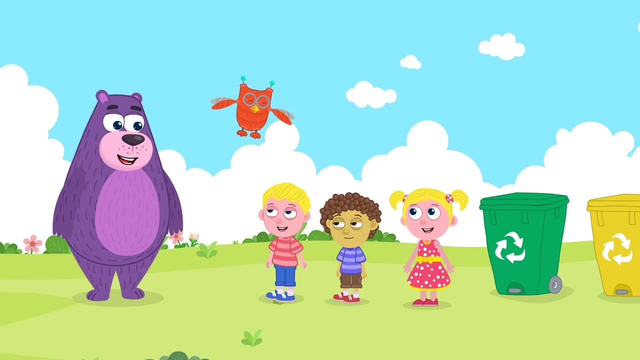 This one is for cardboard, like the tubes the nuts came in, And this one is for plastic, like juice bottles. Looks like you made Momo angry when your rubbish landed on him. Sorry Momo, Sorry Momo, That's better.